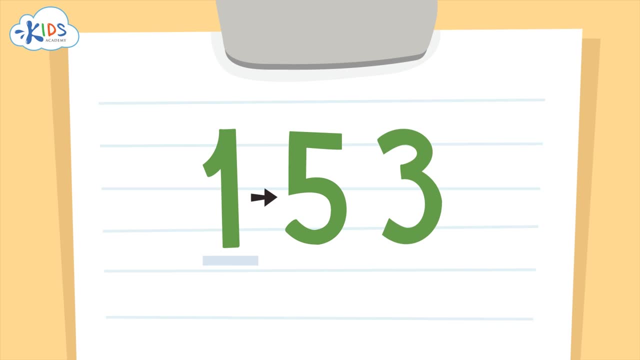 me whether to round up or round down the tens place. You always look one place to the right of the place that you want to round to. So in this case we're rounding to the nearest hundred, So we'll have to look at the place to the right of the hundreds, which is the tens. 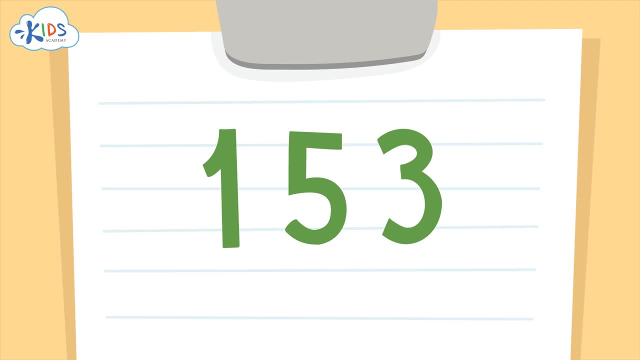 The same rule applies when rounding to the hundreds place as it does when we round to the tens: Five is the key number. If it's five or higher, you round up. Four or lower, you round down. You round the number in the hundreds place and make the numbers in the ones. and 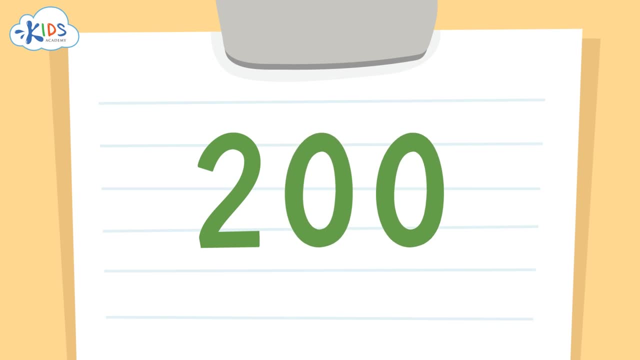 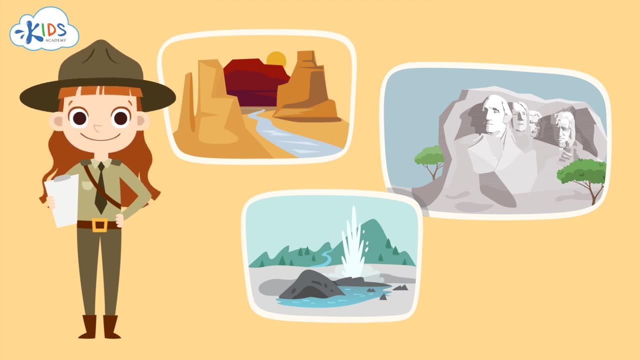 the tens places zeros. Let's take a look at a real life situation that requires rounding and see how our rounding to the nearest hundred skills can come in handy. This park ranger wants to record how many people visited these national landmarks by rounding up to the nearest. 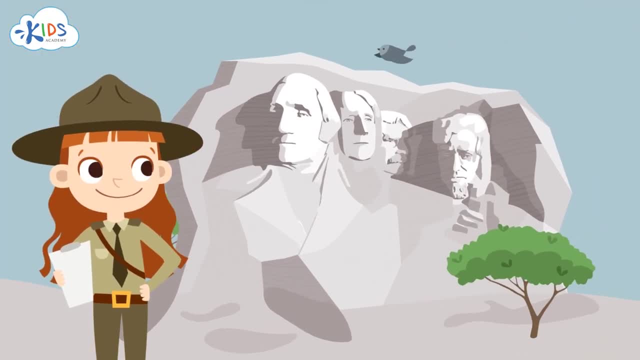 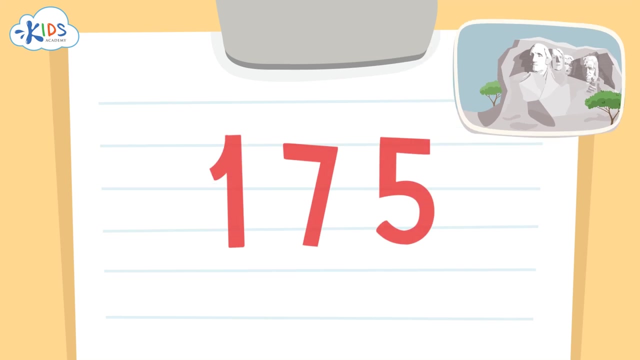 hundred. Let's help her by rounding. First- we'll check out the numbers in the ones and the tens place, One of my favorite landmarks. According to the data, 175 people have visited Mount Rushmore. Now let's round that number to the nearest hundred. We'll use the strategy. 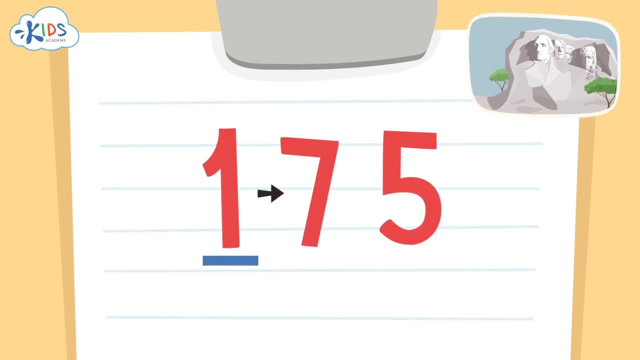 of underlining the hundreds place and drawing an arrow to the tens place so we know what numbers we have to look at. I see a seven in the tens place. I know if it's five or higher. we have to round up. The one in the hundreds place is underlined. 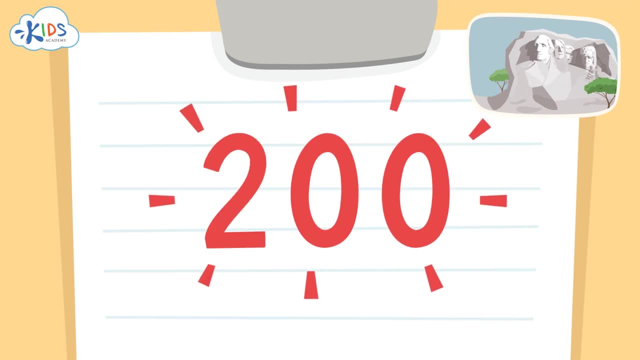 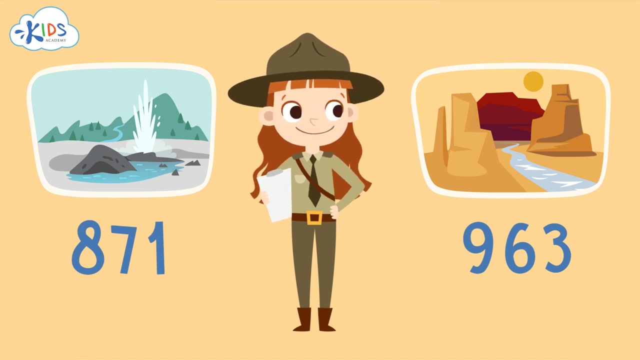 So we'll have to round the 100 up to 200.. When rounding to the hundreds place the numbers in the tens and ones places become zeros. I'll leave you with a challenge. I want you to help the ranger round the next two landmarks. visitors to the nearest hundred I'll give. 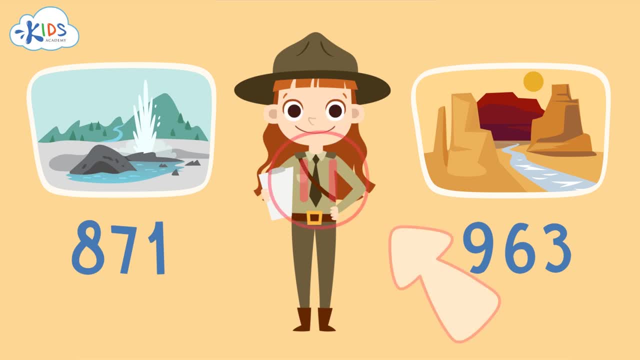 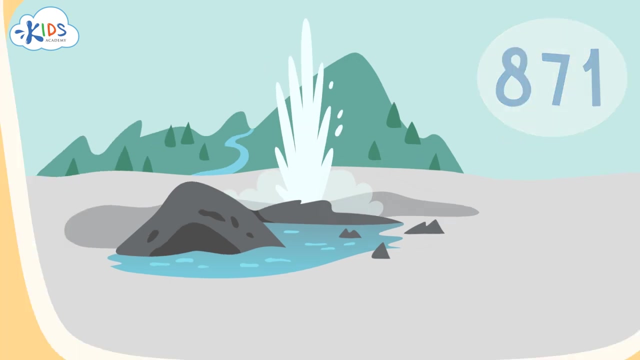 you some time to think, but if you need more time, you can pause the video and answer when you're ready. Okay, here's the answer. Old Faithful saw 871 visitors, So we'll use the strategy of underlining the hundreds place and drawing an arrow to the tens place so we know what numbers we 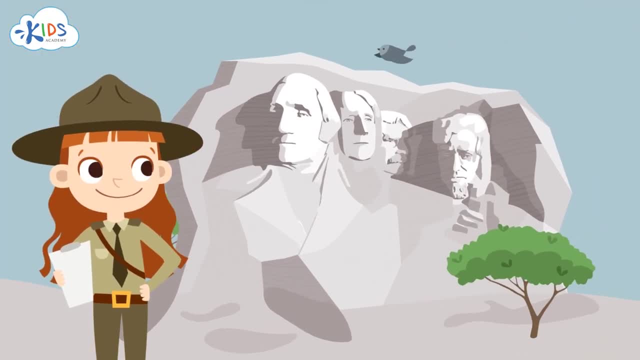 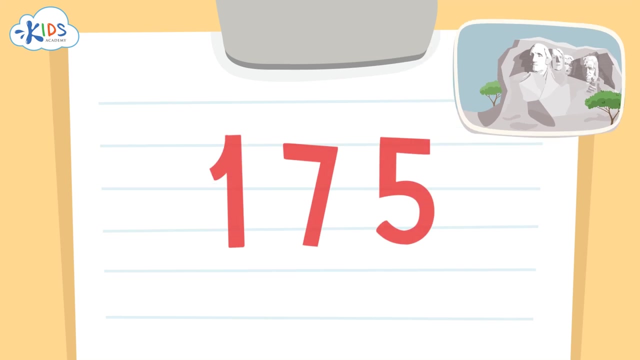 hundred. Let's help her by rounding. First- we'll check out the numbers in the ones and the tens place, One of my favorite landmarks. According to the data, 175 people have visited Mount Rushmore. Now let's round that number to the nearest hundred. We'll use the strategy. 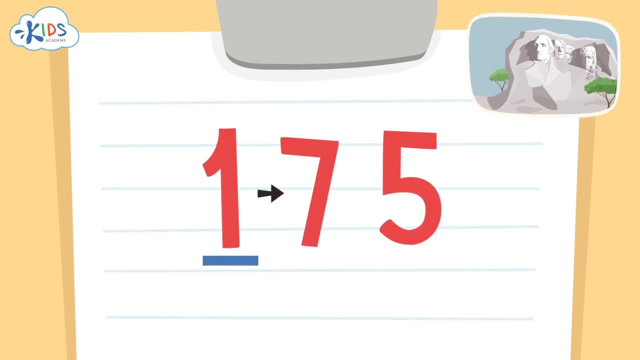 of underlining the hundreds place and drawing an arrow to the tens place so we know what numbers we have to look at. I see a seven in the tens place. I know if it's five or higher. we have to round up. The one in the hundreds place is underlined. 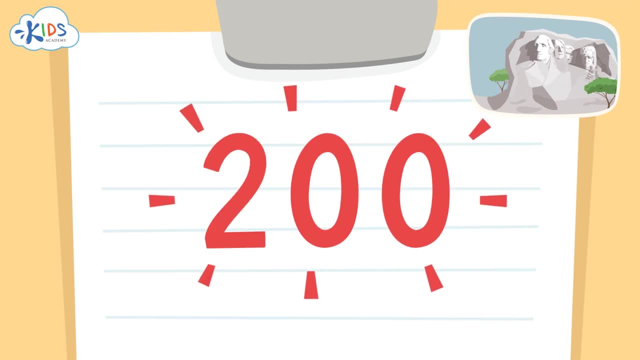 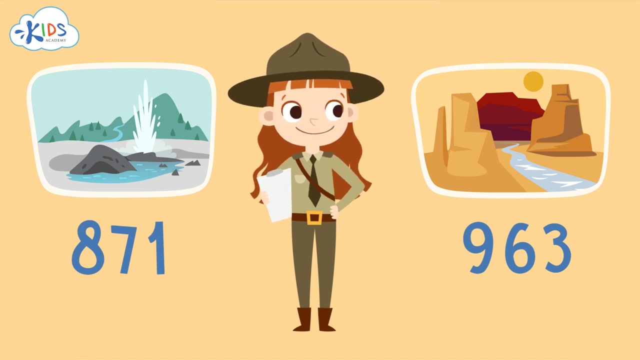 So we'll have to round the 100 up to 200.. When rounding to the hundreds place the numbers in the tens and ones places become zeros. I'll leave you with a challenge. I want you to help the ranger round the next two landmarks. visitors to the nearest hundred I'll give. 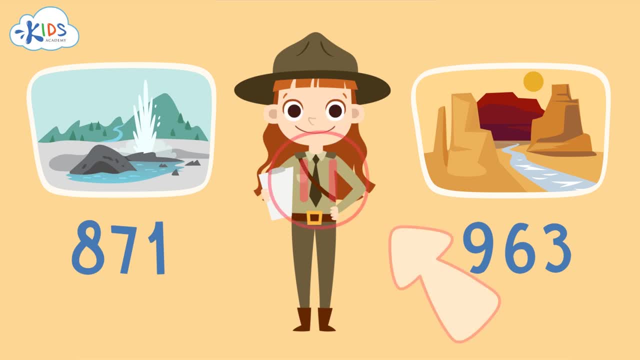 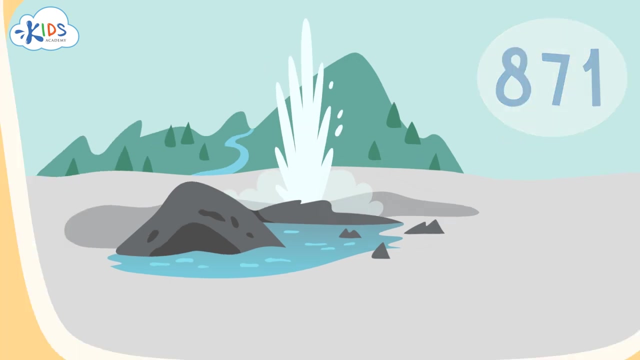 you some time to think, but if you need more time, you can pause the video and answer when you're ready. Okay, here's the answer. Old Faithful saw 871 visitors, So we'll use the strategy of underlining the hundreds place and drawing an arrow to the tens place so we know what numbers we 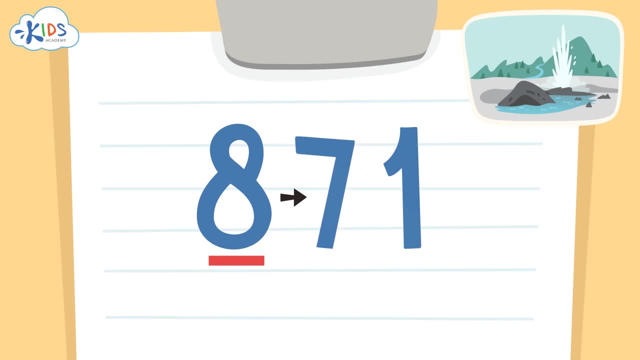 have to look at. I see a seven in the tens place. I know if it's five or higher we have to round up. The eight in the hundreds place is underlined. So we'll have to round up. So we have to round up the 800 to 900.. When rounding to the hundreds place, the numbers, 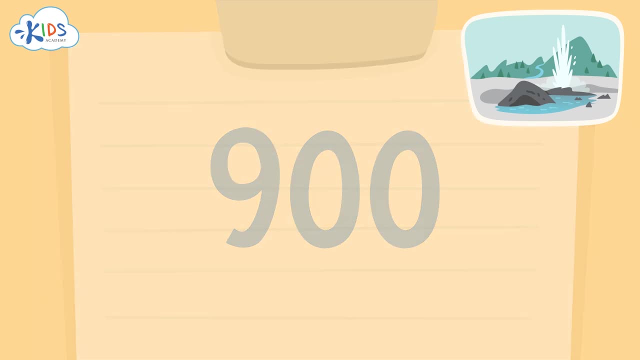 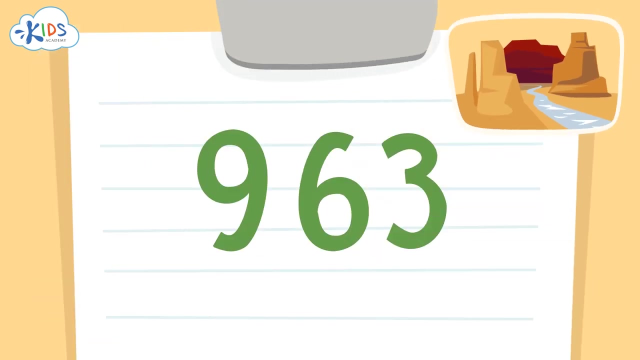 in the tens place and ones place become zeros. The Grand Canyon saw 963 visitors. We'll use the strategy of underlining the hundreds place and drawing an arrow to the tens place again. I see a six in the tens place. I know if it's five or higher. we have to round up The nine. 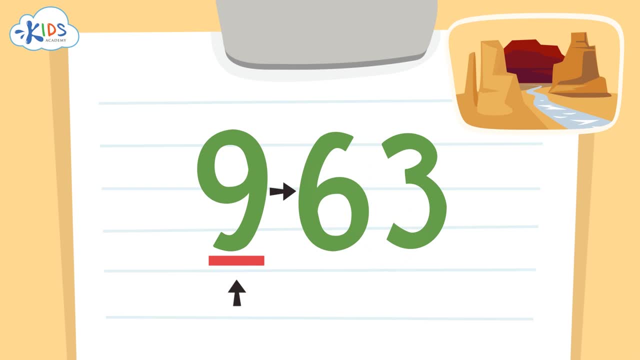 in the hundreds place is underlined. so we have to round up the 900 to 1000, because after 900 we have to change to thousands. When rounding to the hundreds place and we have to round up to a thousands, the numbers in the hundreds, tens and ones place become zeros.